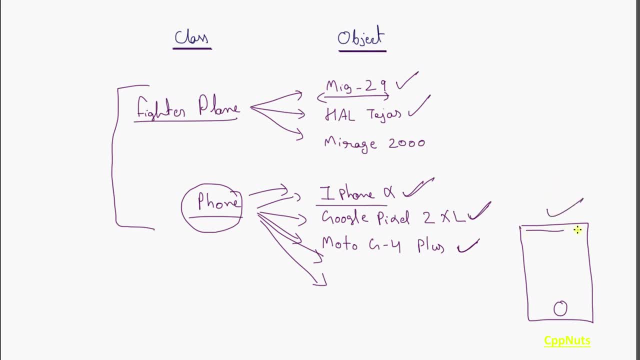 Like the phone should look like this one, and this is going to be the screen part, and here we'll put some buttons and all that. Okay, so the blueprint should be ready in order to actually create That. Okay, so, before you need to create the classes in order to create the object, So first understand what is the requirement for creating the class. There are two things you need to create in class. First is attribute and another one is the functionalities. These functionalities you can understand, like the operations you can perform on the object, Okay, and attributes like how it would look, like Like if it is iPhone or Google Pixel phone. 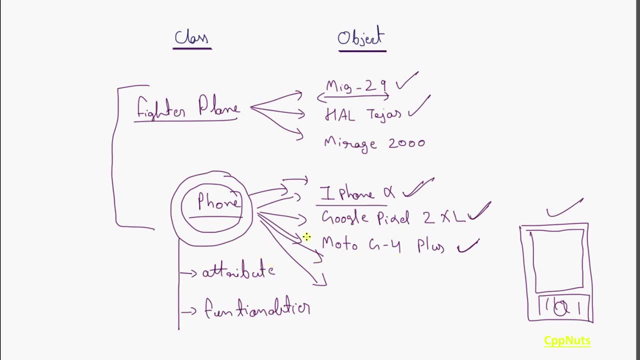 Pixel and Moto G4. Then what will be the screen size and what will be the chipset inside that and all those real attributes of some particular phone. Okay, so you will be setting the attributes and the allowed operations, that, what operations you want to allow to your phone, like receiving a call and watching videos, playing some music and all that. So those are the operations. So let's create the class of phone. We'll understand that a little better. 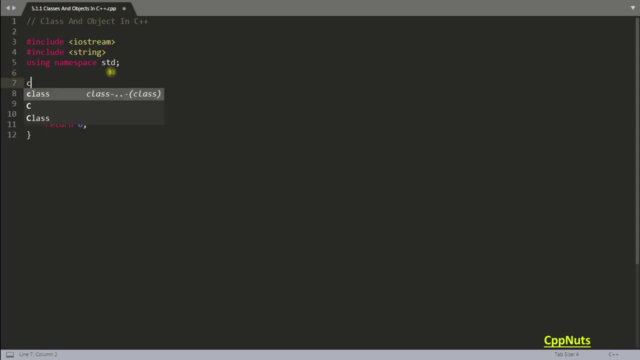 So, in order to create a class, first you need to write a keyword name- class- and the name of the class. So our name goes like this and there are some standards like: if you have written your class name, then the initial character should be an uppercase character. Okay, so this is our class and we'll start with curly and braces and this semicolon. 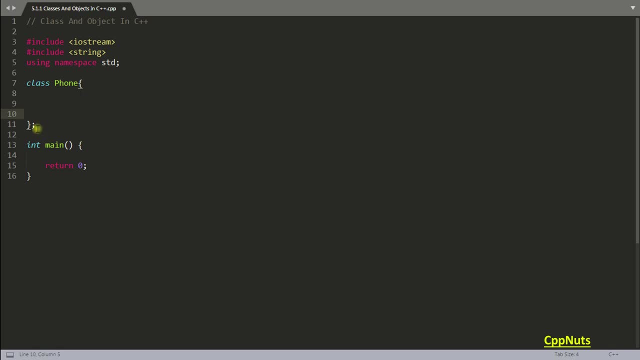 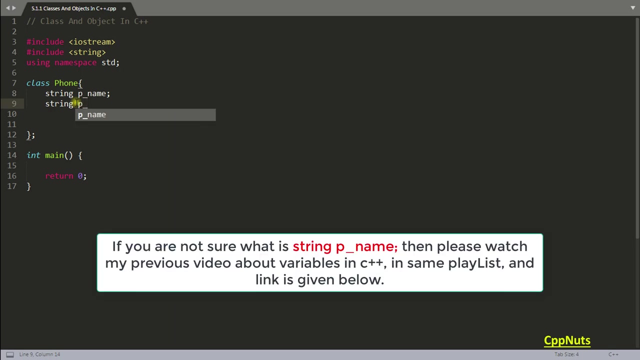 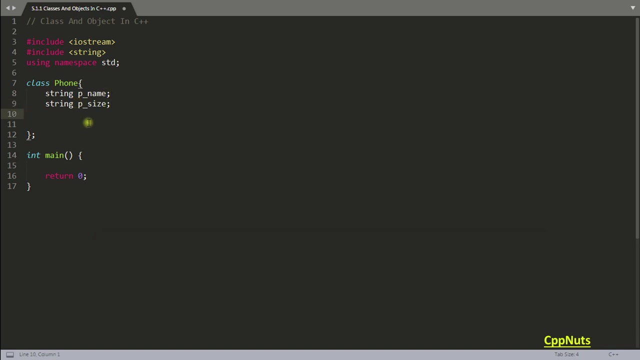 So now, whatever will come inside- This is starting and ending curly bracket- will be considered the part of this class. Okay, so whatever you want to write should belong to your class. You will be writing in between these two. So, as I was telling the attributes, So let's write some attributes. So let's say that phone name, because our phones have name and like size, So some pixel by some picture. Okay, so these are the attributes. You can write as many as you want. 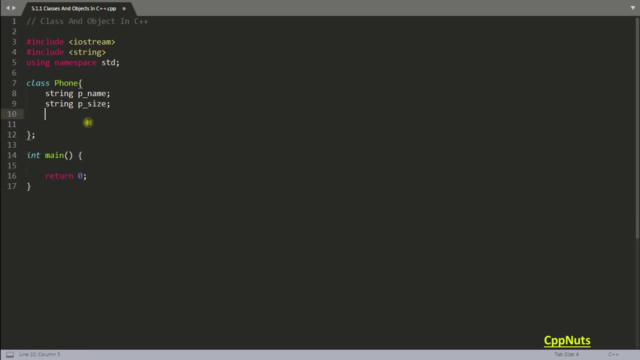 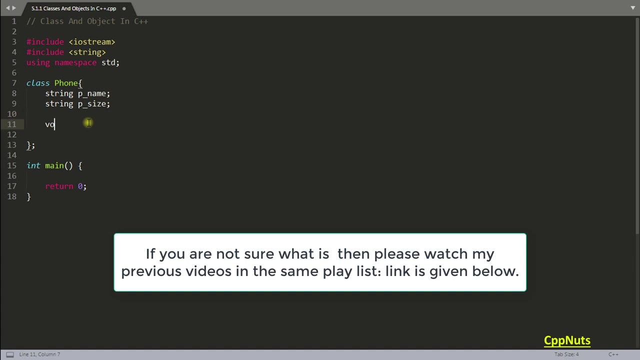 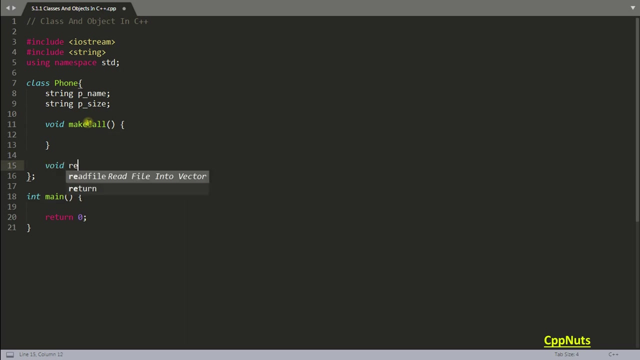 I will be writing these only for the simplicity. and here comes the operations. So operations are called functions in programming language, and operations was like make, make call and another operation could be void- receive, call, Correct. So these two are the operations. Now it's up to you what you want to do inside these functions. and notice this. everything we are writing inside this and 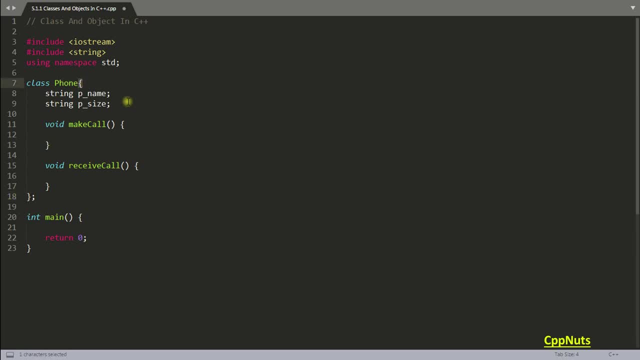 and starting curly braces of our class. So these two are the attributes and these two are the operations. Now here is another thing, something called access specifier. So we have three access specifier: private, protected and public. This is access specifier. I'll talk about later in some videos because that is a big topic. for now You just understand that if you are making something as a public in your class, 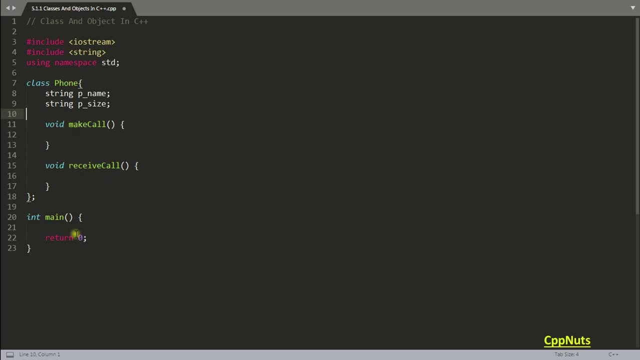 Then you can access that part from outside this class. and if you have made something private, you cannot access that private stuff outside this class. So access specifiers are written like this public. So if you have written public here, it means whatever comes after this is public. So generally we keep the methods or the operations, whatever operations you are making for. 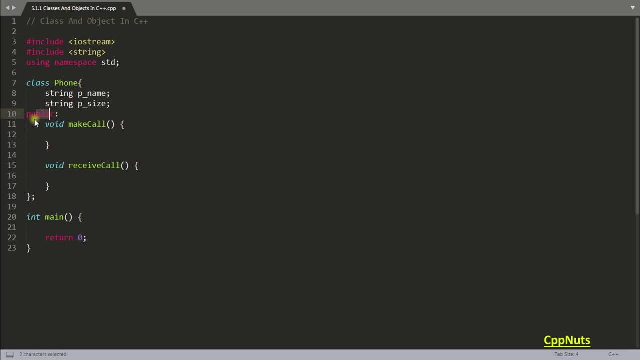 a particular class. we keep all those operations public so that you can call those operations from somewhere else. Okay, Let's print some message which will give you a good idea about this. So making call using this phone, P name, and here we can write like receiving call using the same phone. So till now our two things are ready. First is attribute of the. 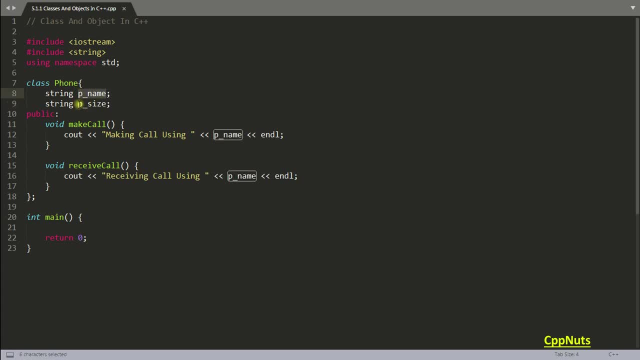 phone like how the phone would look like, what will be the name of the phone and the size of the phone, what chipset will use and all that and what operations are allowed. So for simplicity, I'm keeping just simple operations. So these things are ready. Now there is something called constructor, which is a special member function and used to construct the object. Okay, And this is how the constructor look like. There are two, three types of constructors that we'll discuss later. 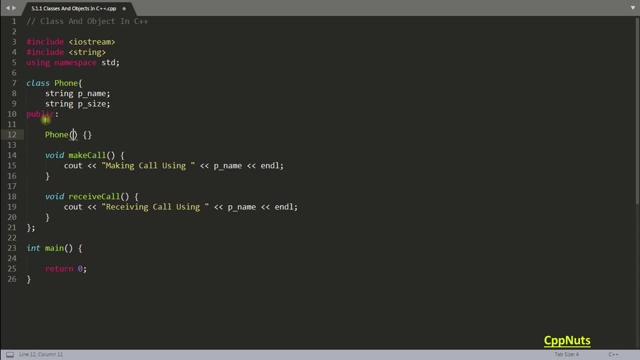 But for now you just understand that constructors are having the same name, what your class name is, and they are used to construct the object. So as this is used to construct the object, it will take some parameters and assign these attributes. So I'll just show you. just bear with me till end. you will be really understanding the logic behind object and classes. So the string type, name and string type. 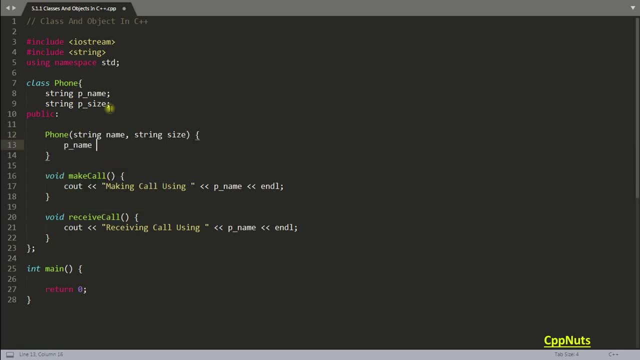 size, and what we will do is p underscore name is equal to name and p underscore size is equal to size. Now we are almost ready. S p percent. So these are the attributes. We generally keep the attributes in private section And yeah, I forgot to mention that you're not writing anything like public, or 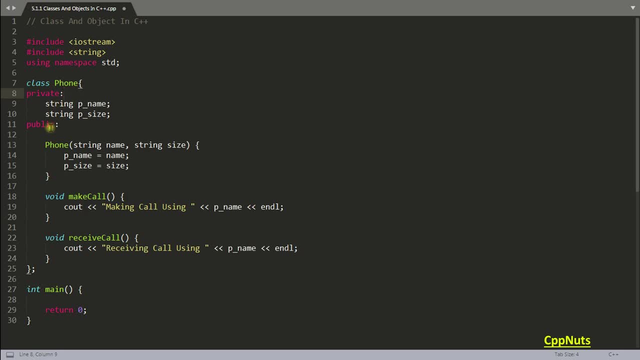 private, Then automatically it will become private. Say before I was not writing this private here. So whatever comes under without any access specifier, that becomes private automatically. So this two lines comes under private section and we keep attributes inside private section so that no one will able to change them without using our own class functions. 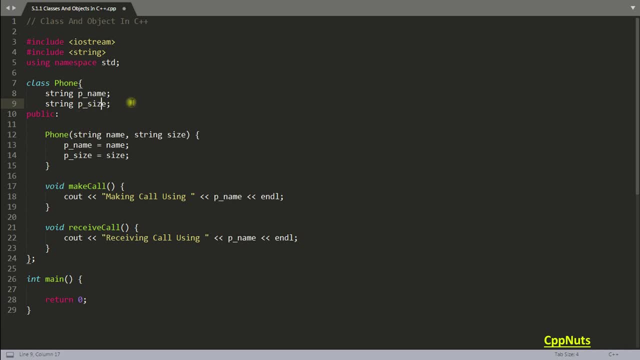 Okay, so that you will see little later. I mean when you will see my whole videos and the full journey of learning C++. we will understand these things by taking the real-time examples. So for now, you just think that these are inside private section and these are inside public. 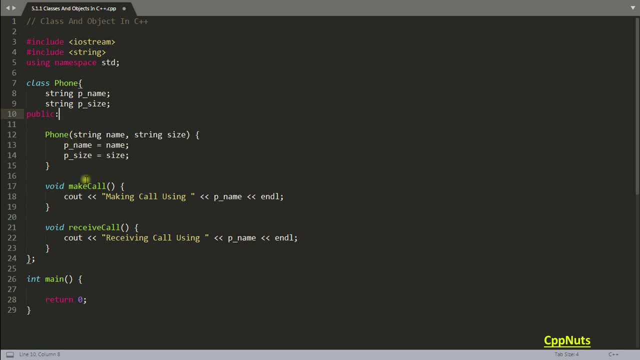 section. So public sections can be called from outside this class. So now let's create an object. To create an object, first you have to write the class name. It will say that what type of object you are creating, and the object name. That could be anything, it depends on you. 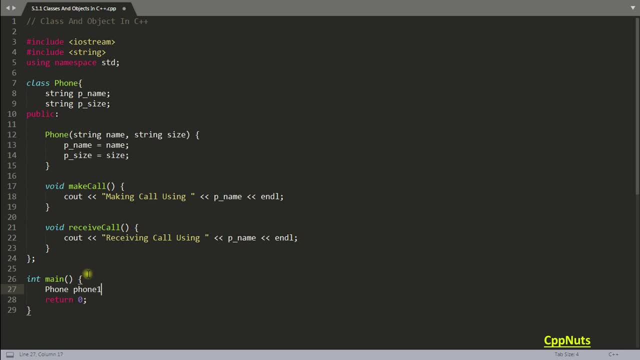 So I will say that phone, Word One: Okay, and you have to pass some parameters, two parameters. So this is where you are going to create a phone and that phone would look like this: Okay, so this is your phone. It is going to look like this and, as you are creating a phone, you will end up calling constructor. 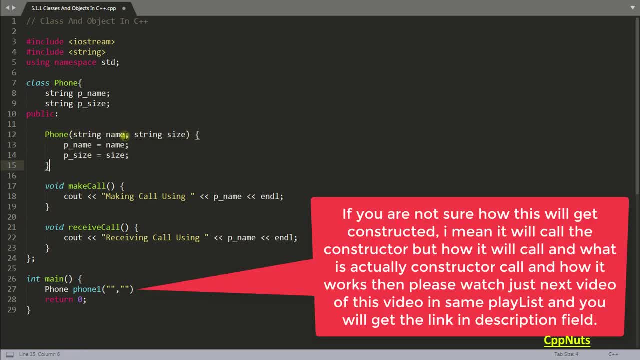 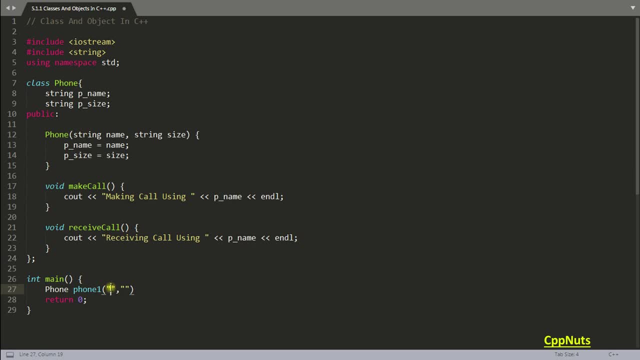 This is your constructor. So, as you can see, if you have some prior knowledge about programming, these are two parameters and here You pass the parameters. So first one is taking the name, So I will just say iPhone X or 10 and, sorry for that, I don't know the pixel size of that. 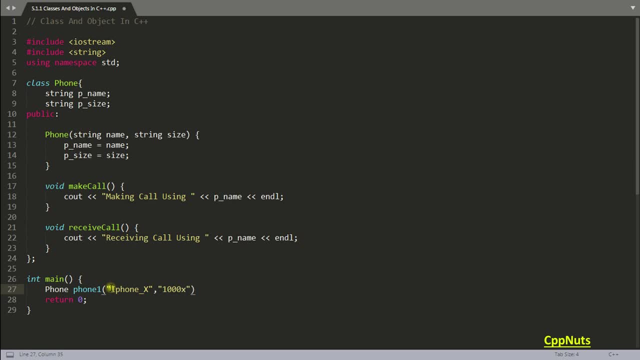 So excuse me for that. I will just simply say that, okay, thousand cross 500. excuse me for this. So actually I am not a big fan of iPhone and phones. actually I am not into phone and all. So your object is ready, Your phone is ready. 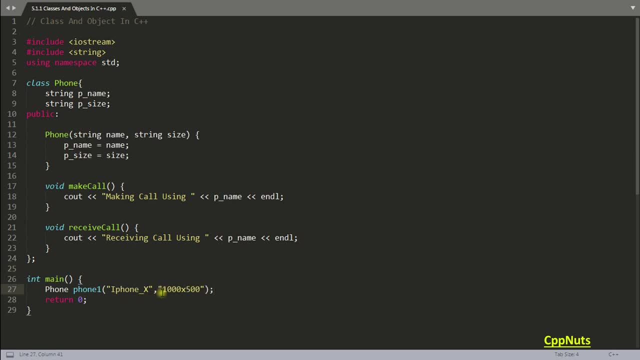 Now, if you want to make some operation on phone- let's suppose you want to call somebody- Let's do that phone make call Now you will get the clear picture. Let's run this see making call using iPhone X. got it. So this is how you perform the operation using your object. 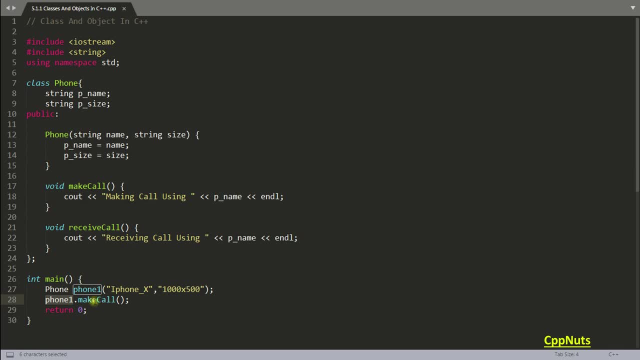 You write the object name dot and write whatever operation you want to do. let's do another operation on the same phone. So phone one receive call. Okay, this is another example and in another function, let's run this: If you are running this receiving call using iPhone X, 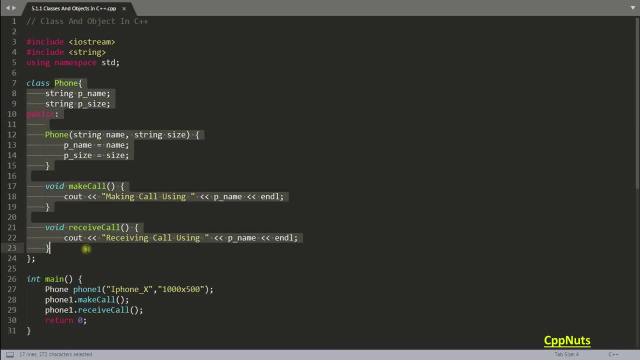 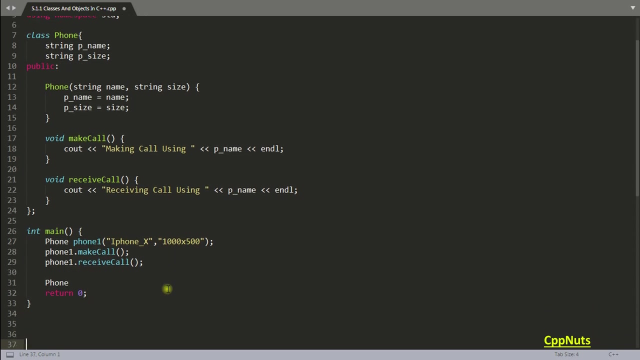 This is the beauty: You have a phone class. These are the attributes, These are the operations, and this is where you construct your phone class. Okay, now let's create another phone. We are creating phones here, man, oh my goodness. So phone class. again, how you create an object. 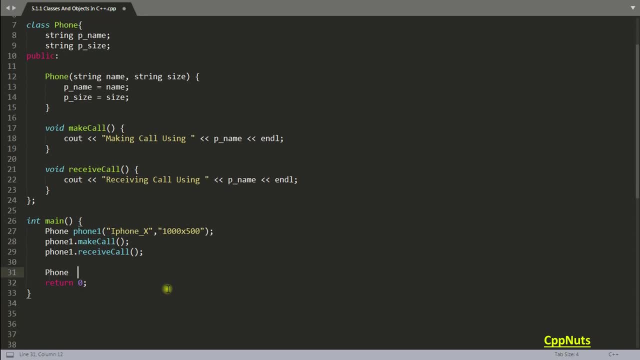 Let me take it to this level and this time we'll say like phone two or something, or you can just give the name some meaningful name so that if someone is reviewing your code they will be able to understand it. So, as this was an iPhone, 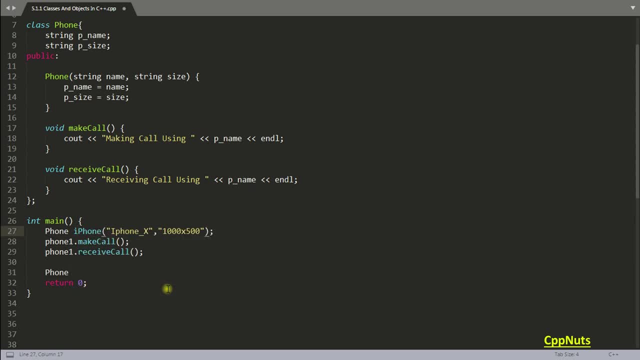 I can say I Phone Okay, and then we have to change: here also iPhone and here also iPhone. So this time, if I will create a Google pixel, then I will be giving like G pixel, and equally I will be passing two parameters here.